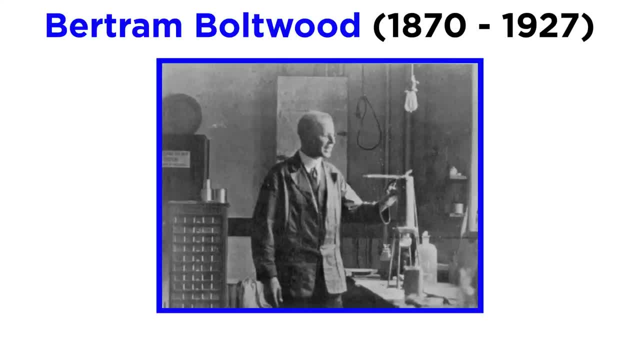 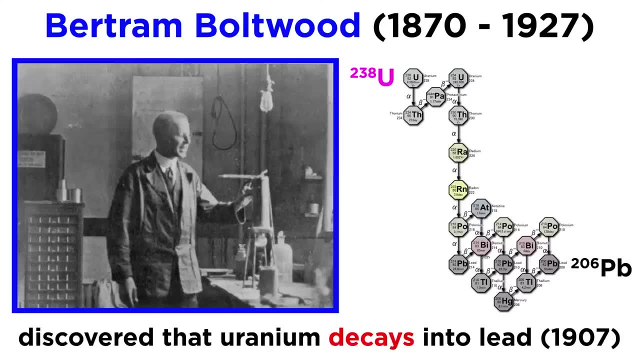 it is highly reliable, so let's learn more about how this works. Radiometric dating was first documented in 1906, and it was first used to date the rock. The rock was first used to date the rock in 1907, by Dr Bertram Boltwood after he discovered that uranium decays into lead. 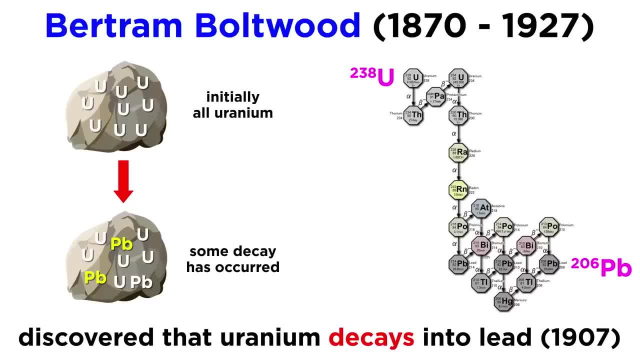 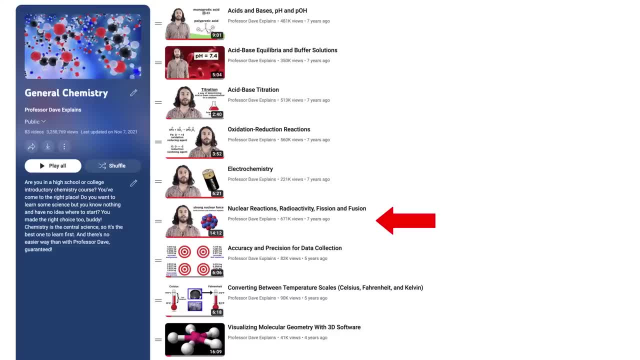 and that the uranium to lead ratio present in a rock would vary based on the rock's age. We've discussed nuclear decay in some detail over in the general chemistry series, so check out this tutorial if you need a thorough refresher on nuclear stability. 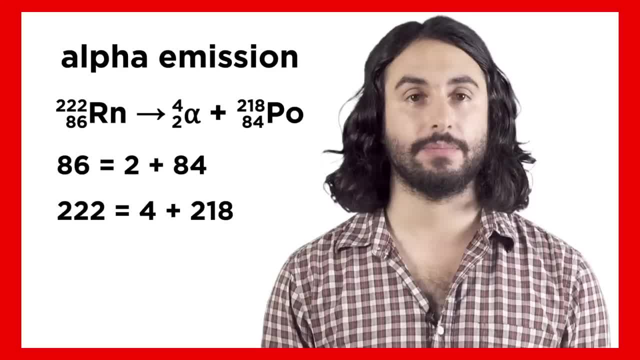 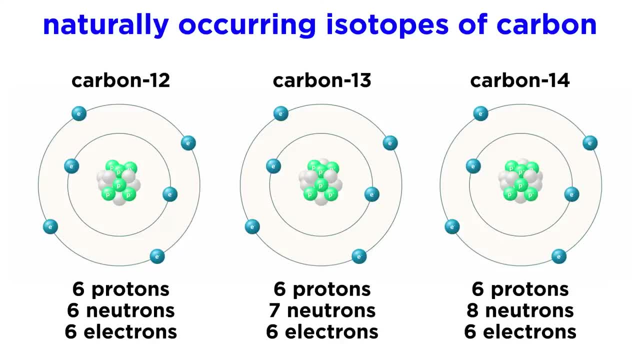 nuclear reactions and applications. Otherwise, let's reiterate the main concepts and contextualize them. The utility of radiometric dating is based on the existence of isotopes or atoms of the same element with differing numbers of neutrons. Carbon, for example, has three naturally occurring isotopes. 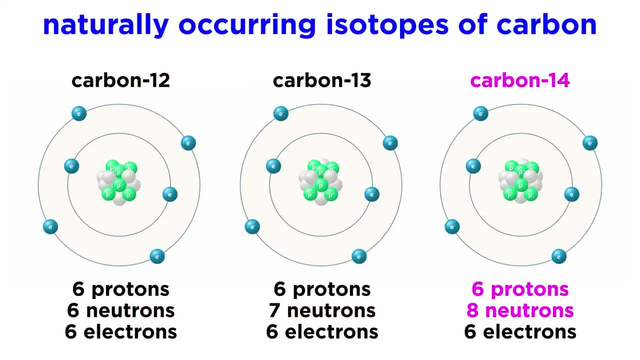 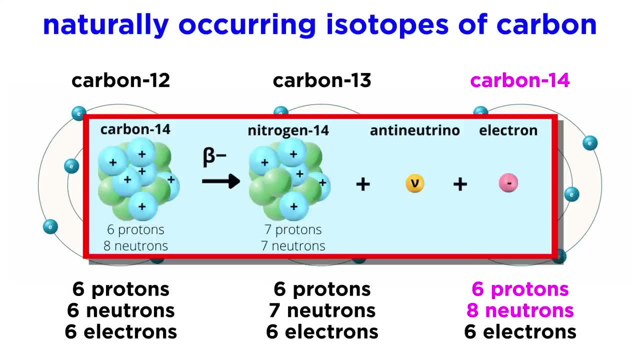 carbon-12,, carbon-13, and carbon-14.. Of these, only carbon-14 is radioactive due to an unfavorable proton-to-neutron ratio. It will therefore break down into nitrogen-14 via beta decay or the emission of an electron, which causes a neutron to become a proton. 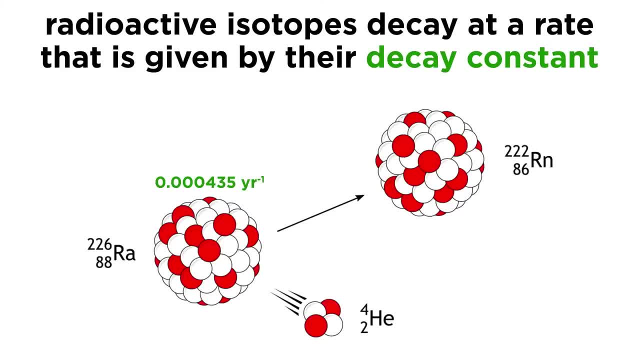 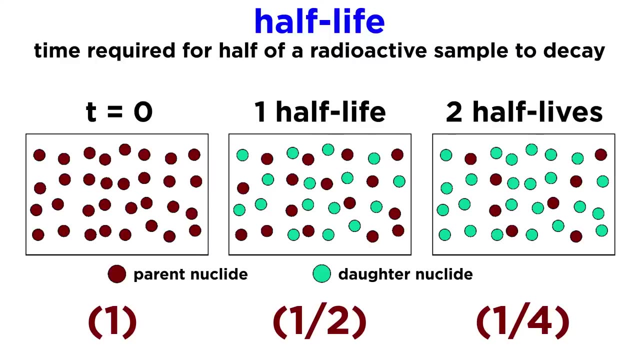 thereby transmuting the nuclide. Radioactive isotopes decay at a specific rate that is represented by the isotope's decay constant or number of disintegrations per year, which can be used to calculate its half-life or the amount of time it takes for half of the radioactive parent nuclide to decay into the. 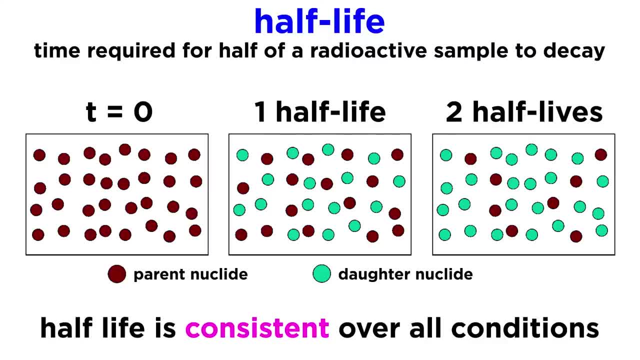 daughter nuclide. The consistency of this half-life is extremely reliable and does not depend on any aspect of the environment. It will be the same everywhere in the universe and under any set of conditions, And because the isotopes of a given element also decay at a specific rate, the 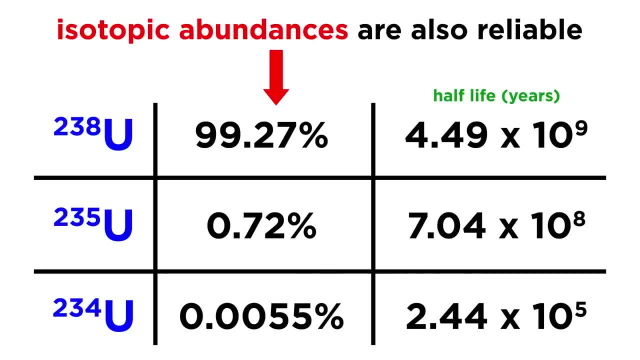 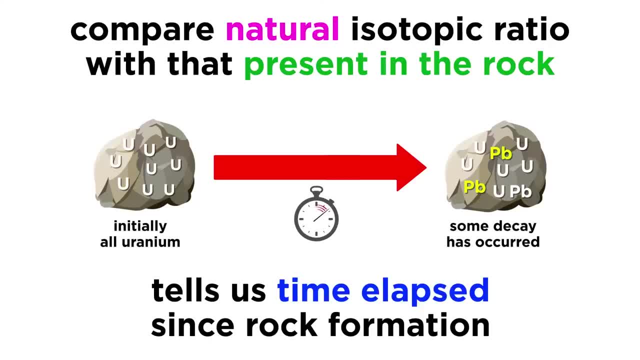 number of times they decay is determined by the atomic mass. So if we have a very reliable natural abundance which we use to determine atomic mass, it is a relatively straightforward matter to compare some isotopic ratio in a particular geologic material with the naturally occurring. 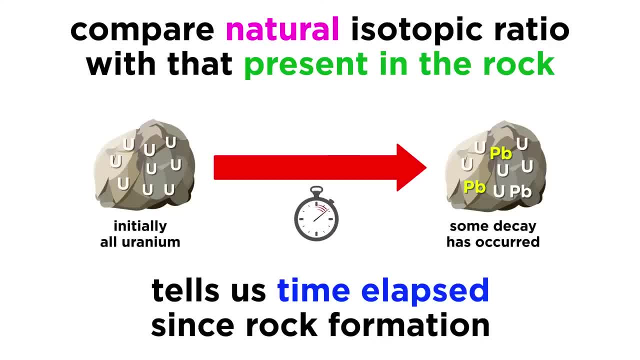 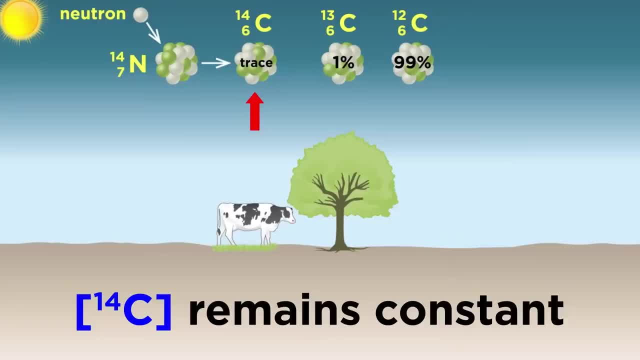 ratio in matter which is being formed and freely exchanged with its environment, like the way that carbon-14 is produced by cosmic rays from the sun and maintains a nearly constant concentration in the atmosphere. This comparison allows us to determine how many atoms are in the atmosphere and how many atoms are in the atmosphere, So if we have a very reliable 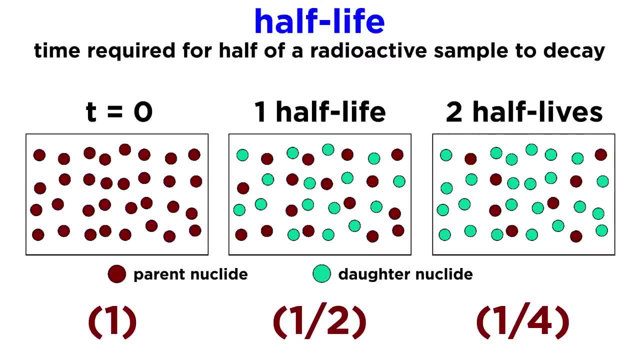 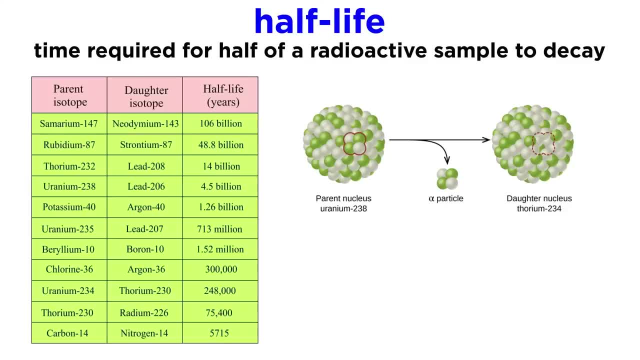 representation of the atomic mass, we can determine how many atoms are in the atmosphere and how many half-lives have elapsed, and therefore the age of the object. Each radioisotope has a unique time period over which it is useful for dating, which is related to its half-life, Namely the parent. 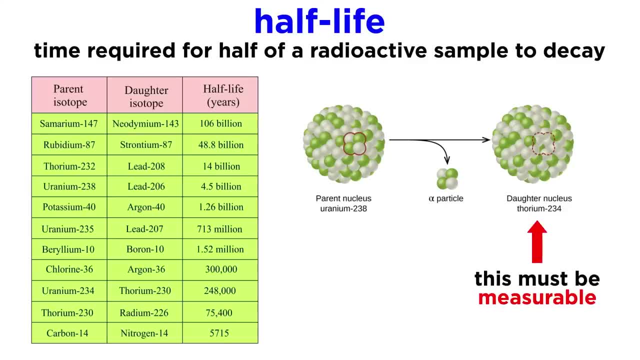 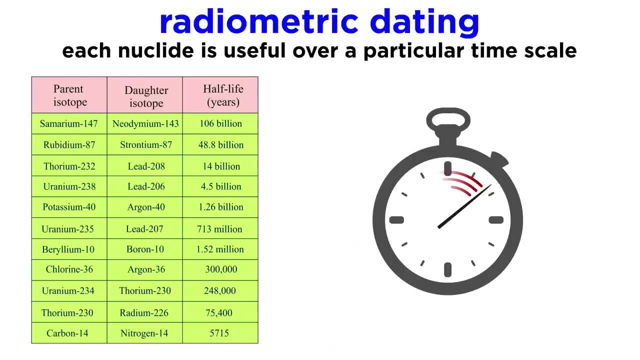 must have decayed enough to produce a measurable amount of the daughter isotope, but not so much that the parent has almost totally disintegrated. Here are a few of the most commonly used parent- daughter pairs and the ages over which they are useful: Carbon-14 and nitrogen-14.. 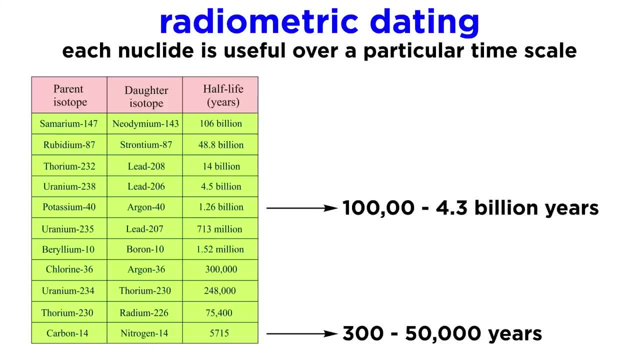 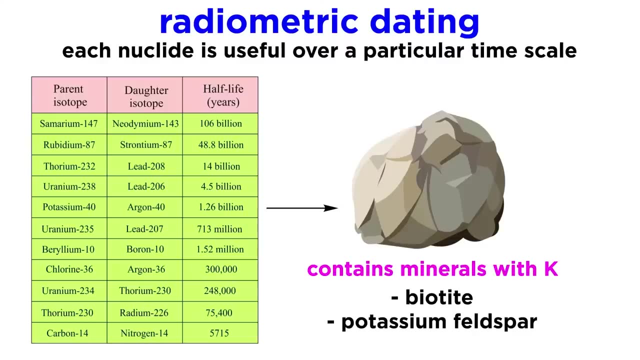 300 to 50,000 years Potassium-40 and argon-40.. 100,000 to 4.3 billion years Uranium-238 and lead-206.. 1 million to 4.5 billion years Potassium-argon dating is used to date rock. 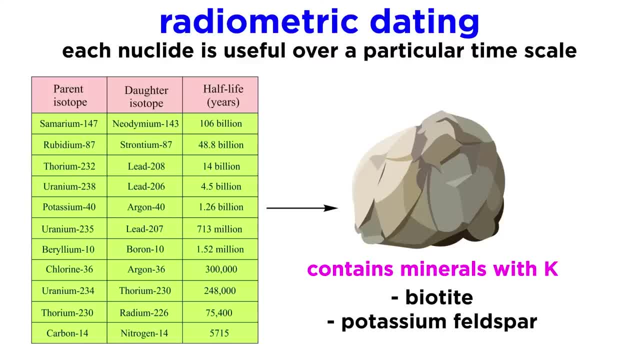 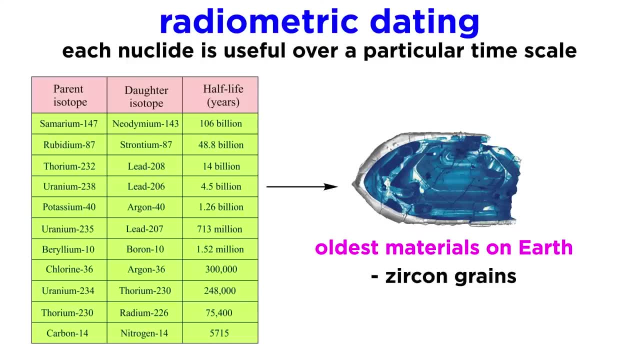 with potassium-containing minerals such as biotite and potassium feldspar. Uranium-lead dating is often used to date the oldest materials on Earth, primarily because of these old materials are almost exclusively zircon grains, which take up small amounts of uranium. 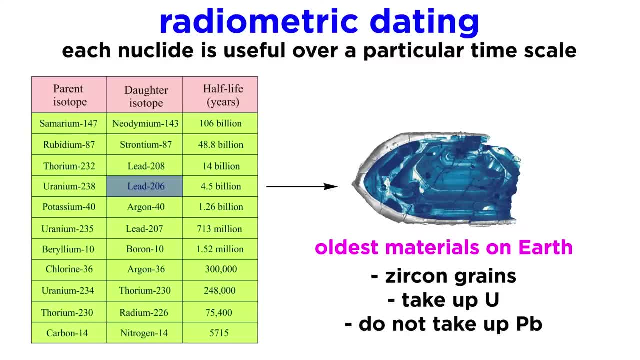 but do not take up lead, meaning that all the lead which can be found in zircon accumulates by the decay of uranium. This is an important assumption that must be made in order to do some types of radiometric dating, which is that the material being analyzed did not contain any isotopes of 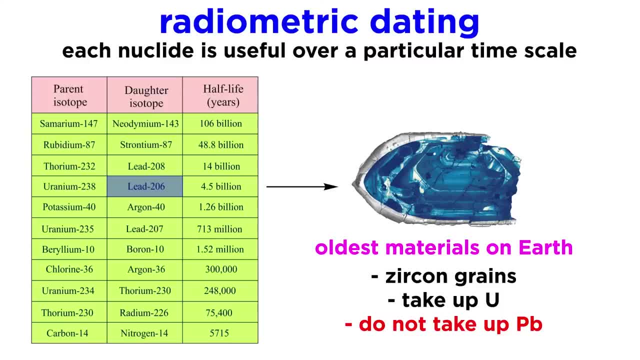 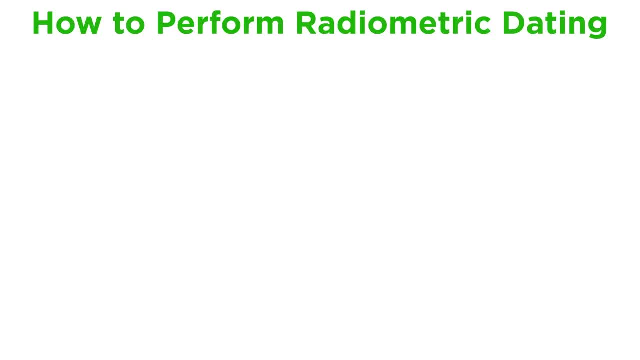 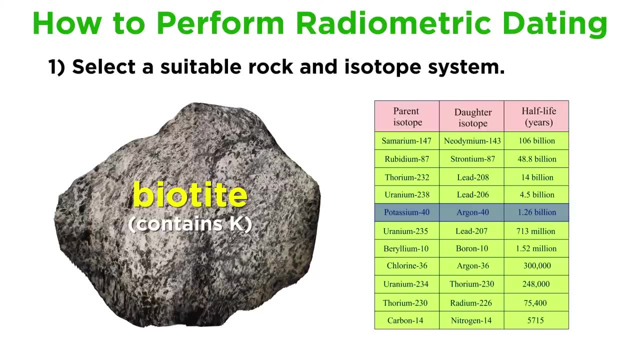 the daughter element at the time it was crystallized. However, isochron dating does not require this. Let's now go over how the radiometric dating process works. First, a suitable rock and an isotope system must be chosen. Let's say our hypothetical rock contains biotite as its only. 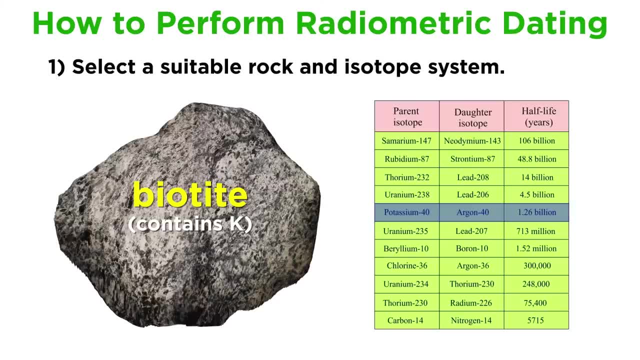 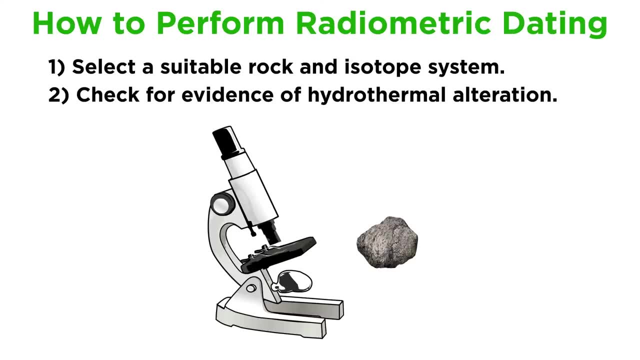 source of potassium, so we will use the potassium-argon system. Geologists must then check the rock's minerals with a microscope to ensure that the rock has not been hydrothermally altered in any way. The sample is then analyzed by a mass spectrometer to determine the amount of radiogenic. 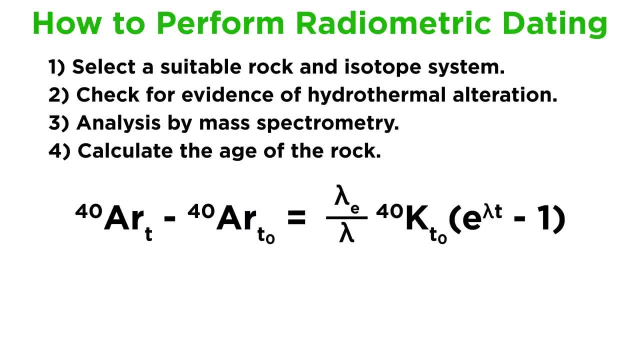 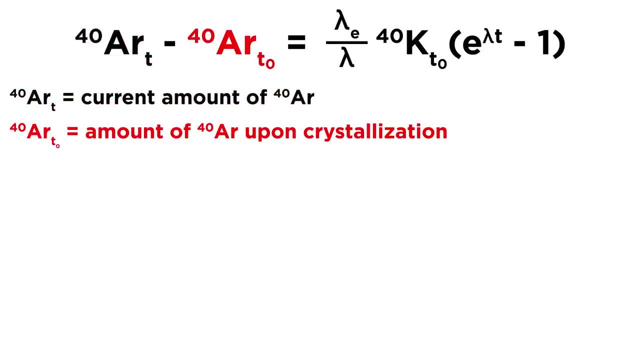 which can then be used to calculate the age using the following formula: where 40rT is the current amount of radiogenic argon, 40 aRT nought is the amount of argon-40 at the time of crystallization. 40 T-naught is the amount of potassium-40 at the time of crystallization. 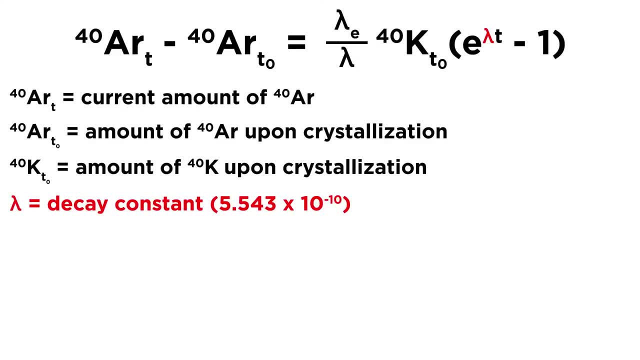 lambda is the decay constant, which is 5.543 times 10 to the negative ten, and lambda-E over lambda is the fraction of potassium-40 via electron capture, which is 0.1048, as potassium-40 can also decay to calcium-40. 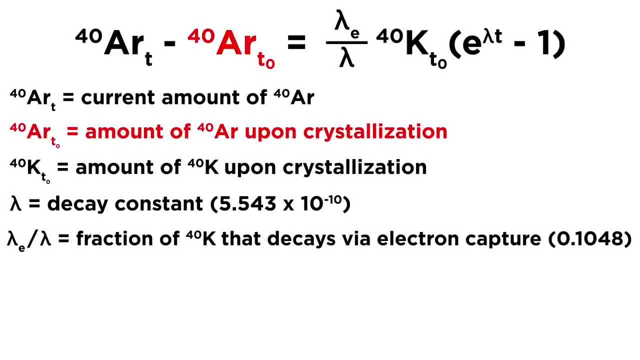 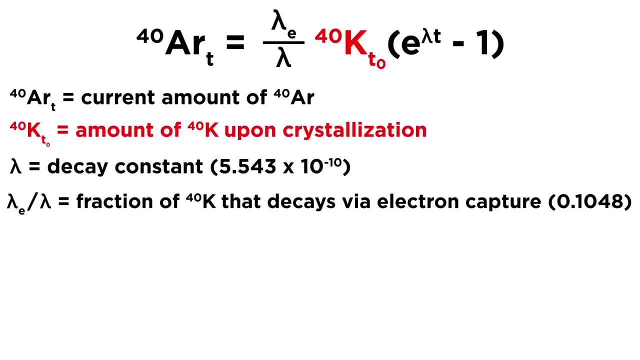 through beta emission. Next, because argon is not taken up into biotite during crystallization, we can assume that 40ArT0 is 0.. We can also calculate 40KT0 simply by knowing the amount of potassium in biotite, which is 4.49×10⁻⁴ moles potassium per gram biotite and multiplying. 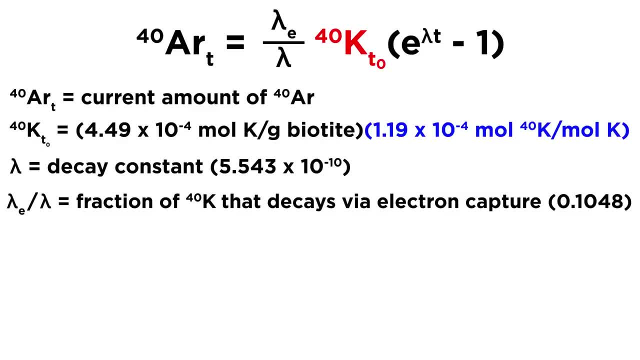 it by the fraction of potassium-40 in nature, which is 1.19×10⁻⁴. After rearranging the equation, we arrive at this, and we can now solve for T, A rock that contains 5×10⁻¹⁰ moles of. 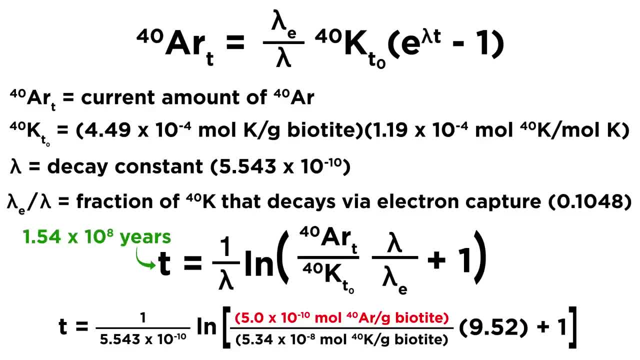 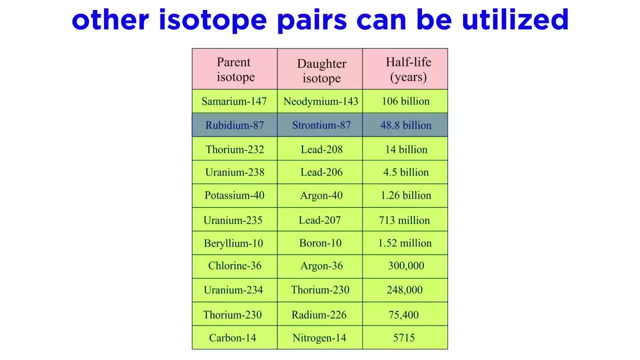 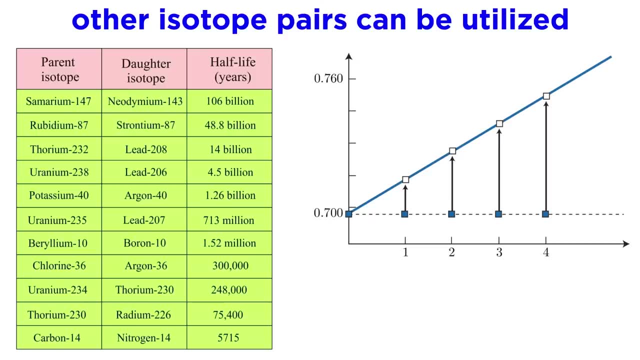 argon per gram of biotite would have a radiogenic expression. There are other isotope pairs, such as rubidium-strontium and uranium-lead, where age is determined by analyzing the relevant isotopes of each mineral of a rock and graphing them In the 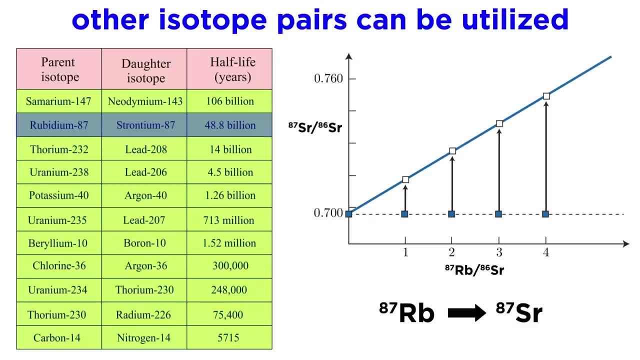 case of rubidium-strontium. rubidium-87 breaks down into strontium-87 through negatron decay, another way of saying beta emission. Here rubidium-87 is the parent isotope, strontium-87. 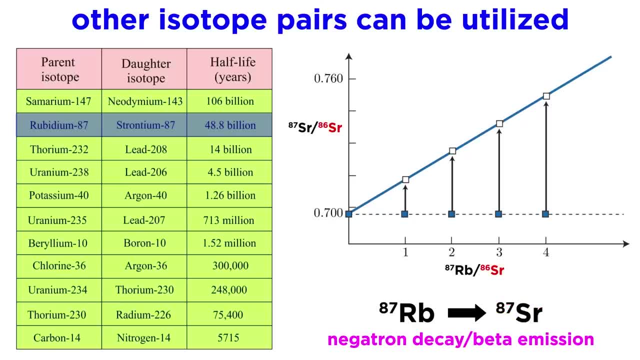 is the daughter of strontium-87, and strontium-87 is the parent isotope. Making a graph with the strontium-87 to 86 ratio on the y-axis and the rubidium-87 to strontium-86. 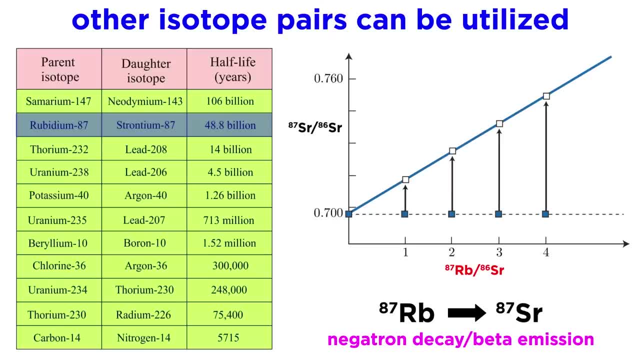 ratio on the x-axis and plotting the values for the various minerals contained in the rock creates a straight line called an isochron. Steeper slopes indicate older samples where more decay has occurred over a long period of time. The exact age can be determined by dividing the slope of the isochron by the decay constant.